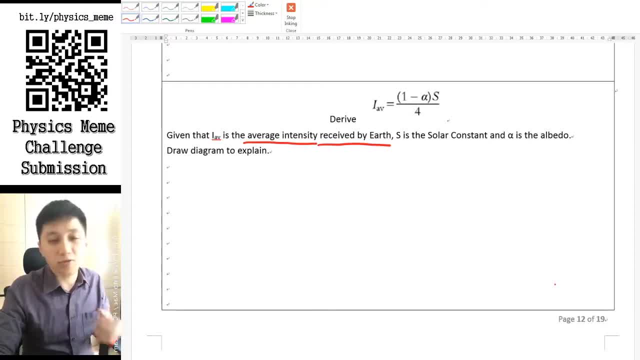 will be very likely required to derive it in the exam paper. so for sure that you want to remind yourself and YouTube with ihspion study about how you can do this, because it is quite popular. before I let you try derive it at yourself, I will need to give you some hint and explain certain terms. firstly, for s, 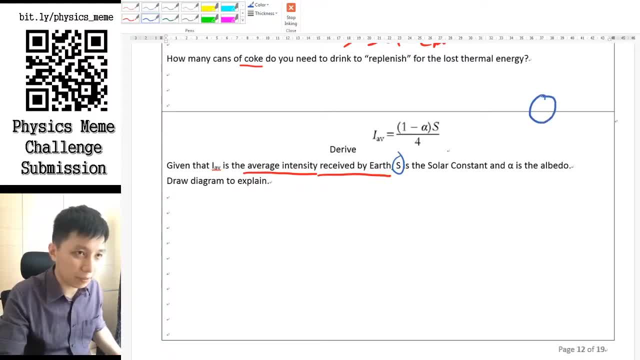 referring to a solar constant it is talked about, for example, if earth is here and the sunlight is going out unbelievable, and that supposedly because it's so far away, so it should be parallel light. but at the same time, let's not forget, we have atmosphere all right around the earth. so 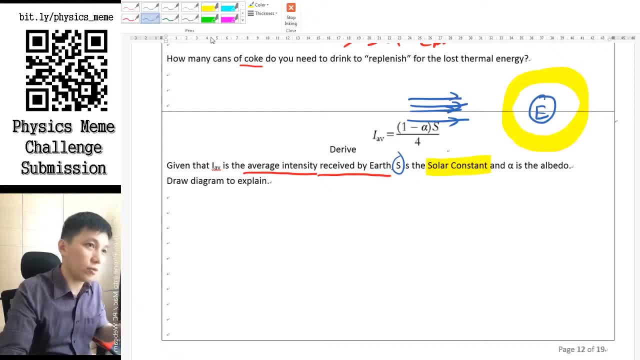 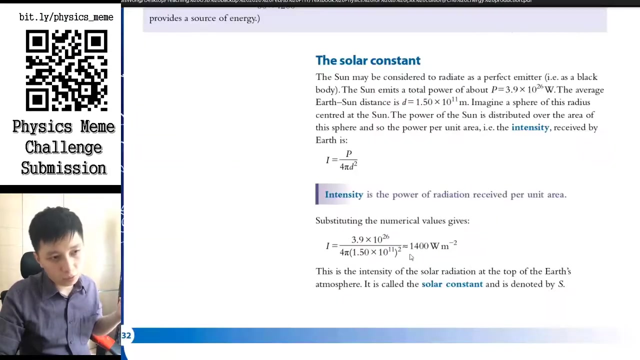 the solar concert here is referring only to the intensity, so that means it is in watts per meter square already for that particular intensity before going through the atmosphere. so on your textbook you can see how you can derive it and it should equal to 1,400 watts per meter square and similarly on the 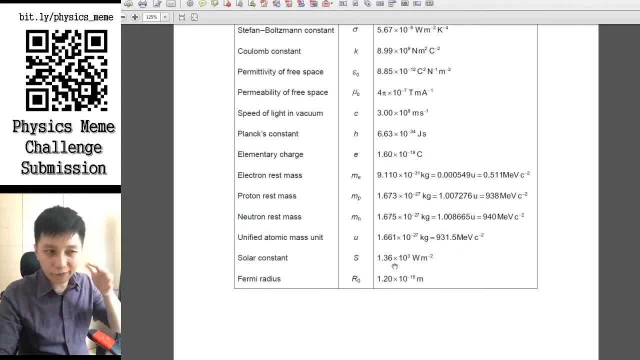 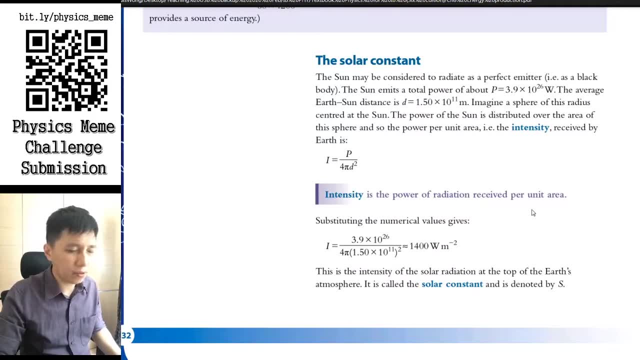 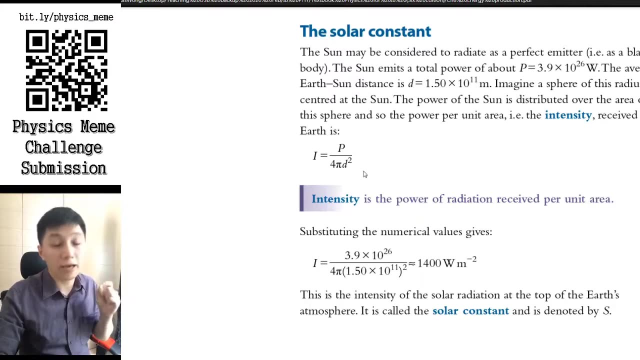 data booklet you also find this number solar constant, roughly also 1,400 watts per meter square. so if you really want to know how this was found, then it's basically by the fundamental definition of intensity, which is, I, equal to P over A, and here the A is actually referring to the spherical area that the Sun can. 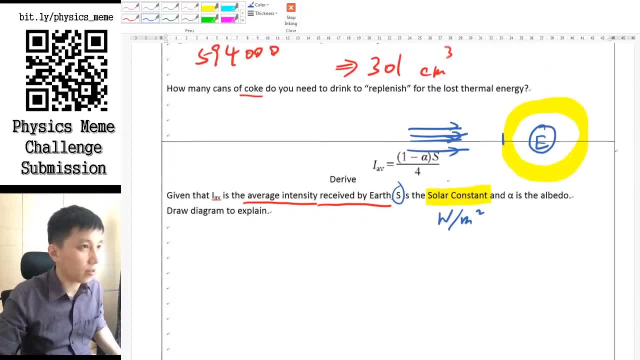 produce. so if I try to draw the diagram then I can do this. I imagine Sun way big of course, way, way bigger, and so when lights can travel through for a certain time, then in all direction of course, then it can cover up to a way bigger sphere. okay, again, this is 2d only, but 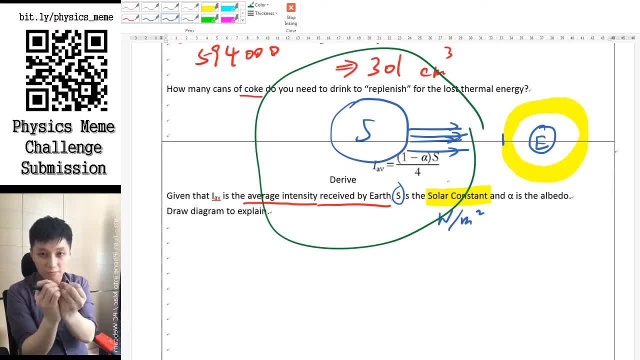 in 3d is gonna be a sphere when light is going to be emitted for a certain time. so imagine a very slow motion of laser got showed out in all direction. then all the laser that come up with will be like a sphere. okay, and so by the time you 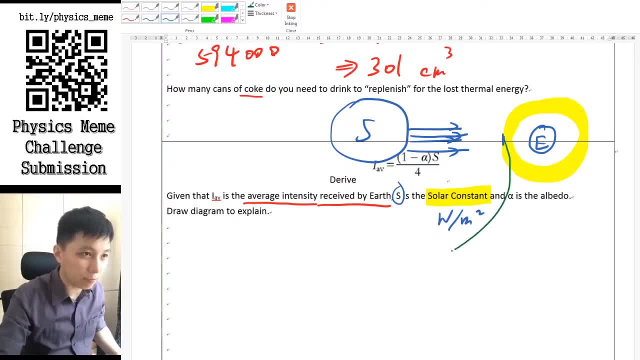 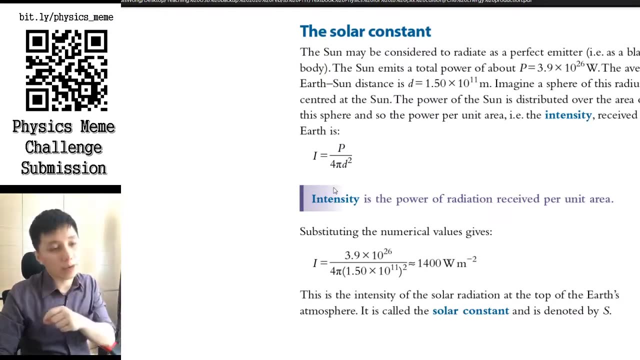 reach to the earth, this fear will become as probably something like this, but again, this is not in scale, of course. okay, and so that's why we have to divide in your textbook here: divide 4 pi D square, because 4 pi L square is the surface area of the sphere and D is a distance between the Sun and the earth. 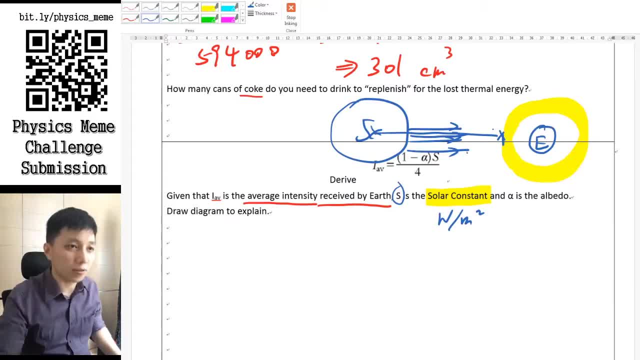 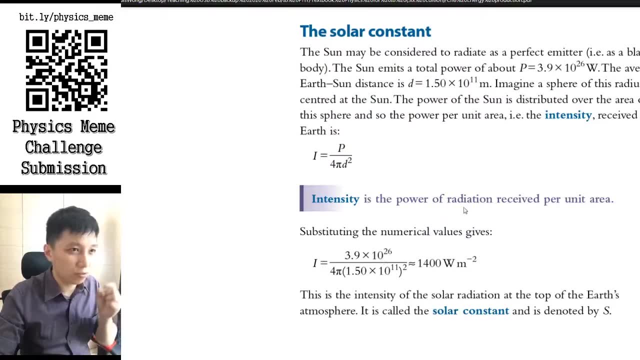 okay, like this one. okay and well, in theory I think it should actually be to the earth center, but since we are talking about to the atmosphere, then I don't know right. it's an average of distance, is that much? actually? I don't think the thickness of the atmosphere matter a lot in this order of magnitude. 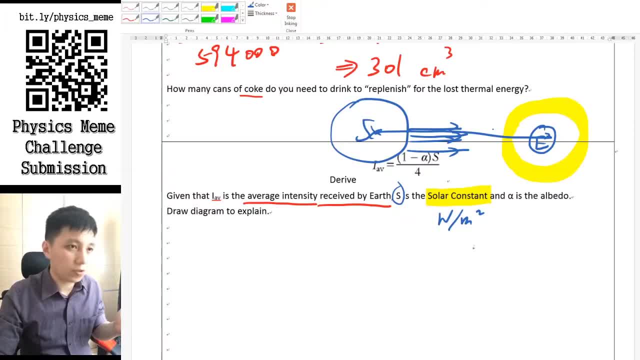 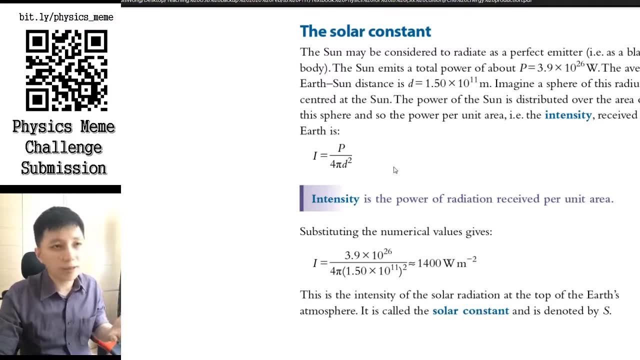 so we can just simply ignore that. so that is why you get the 4 pi D square and somehow, for some reason, that could be explained by another video that people know. the sun's power that is being emitted is 3.9 times ten to the power 26. 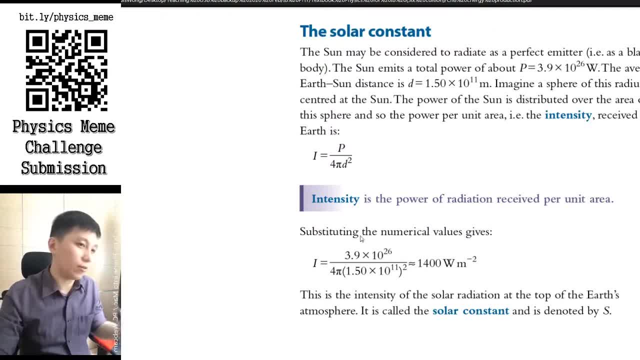 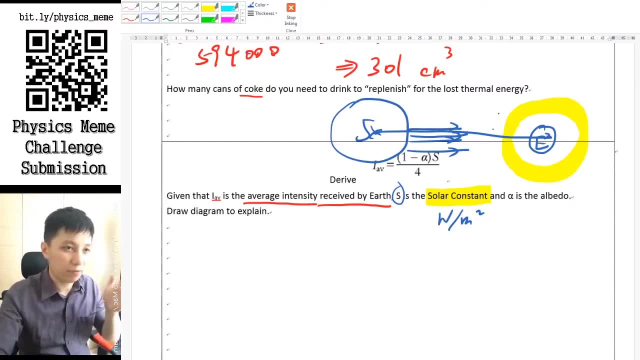 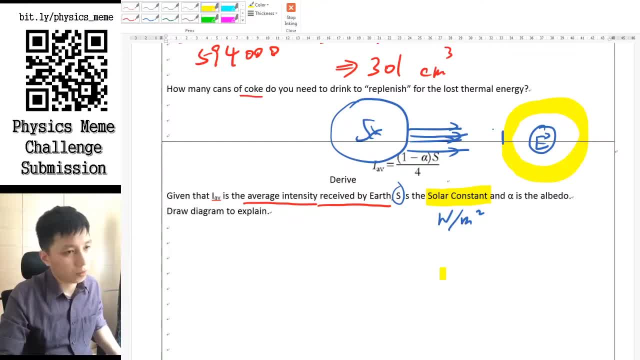 only talking about the top of the atmosphere, only the one that we want to derive is the average intensity received by the earth. so they should say, after it has gone through to the atmosphere, then on the unit area of the earth, then how much intensity that it is receiving. so lastly, there's one more thing that 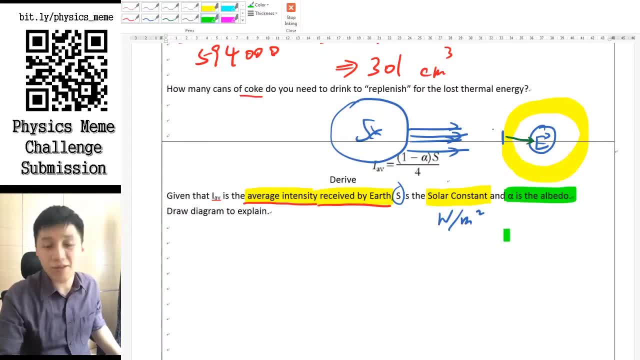 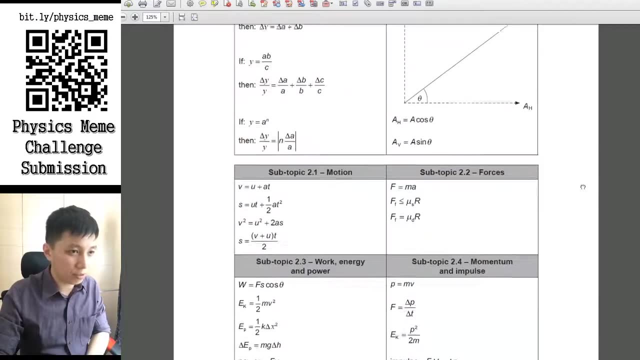 you don't know probably it's called alpha in terms of symbol, here is referring to a word called albedo. albedo is simply referred as the ratio of how much is being received by the atmosphere and how much is being received by the reflected. so you can see in your data booklet in chapter 8.2, right here you can. 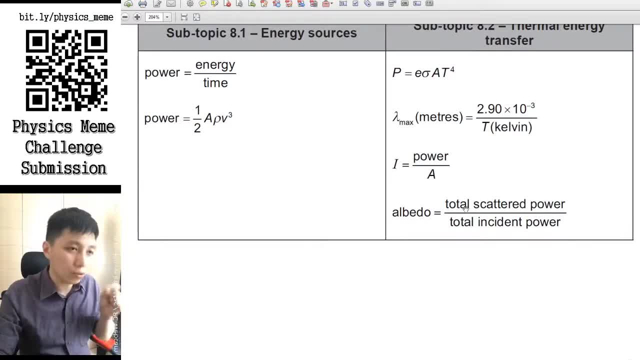 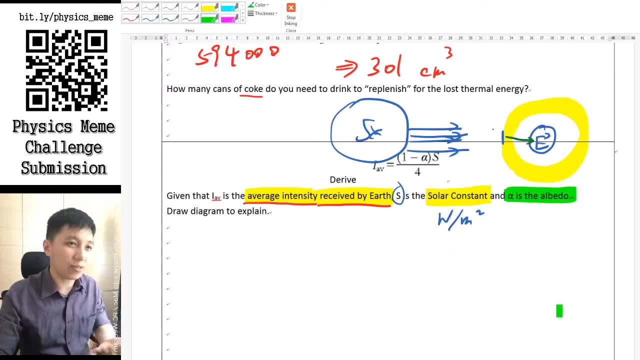 see the so-called definition here: albedo equal to total sketch power over total incident power. so what you can perceive right now is how much of the light intensity are being reflected basically. so it's a bit similar to efficiency: how much is being reflected on how much being? 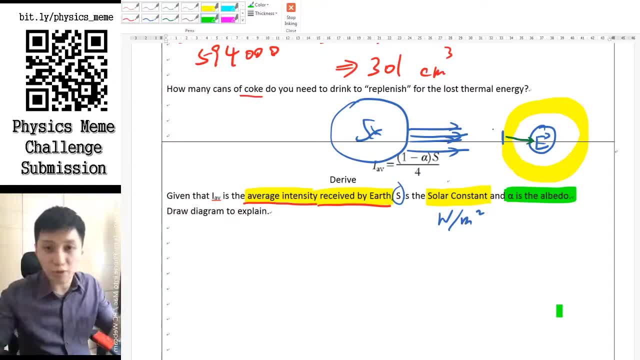 being reflected is mean. so from here, nothing is reflected. much of this isety, as I've said here, so we can see that it's aатьam kubla as means that i'm going to take an economical used in a useful way. One interesting thing that you can write down somewhere on your note. 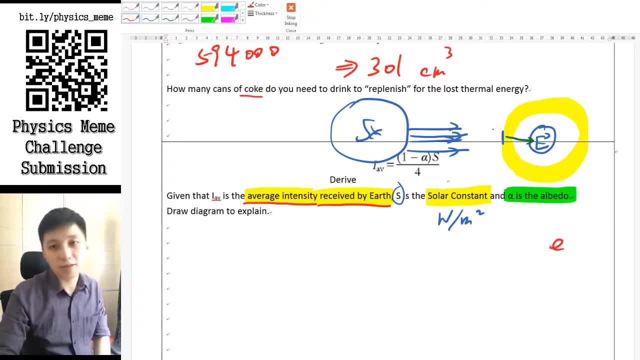 is that earlier we talked about emissivity. Emissivity is how much of light you could effectively absorb and re-radiate again by the body. And here, for alpha, for albedo, the light was simply reflected away, so there's no absorption here. 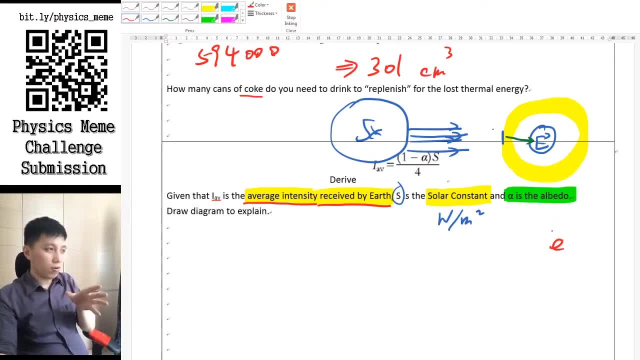 And so for the ratio of albedo and emissivity they actually have a relationship that is not spoken in the test book or even the IP syllabus. So that's gonna be: D plus alpha equals to 1, or you can do it as 1 minus E equals to. 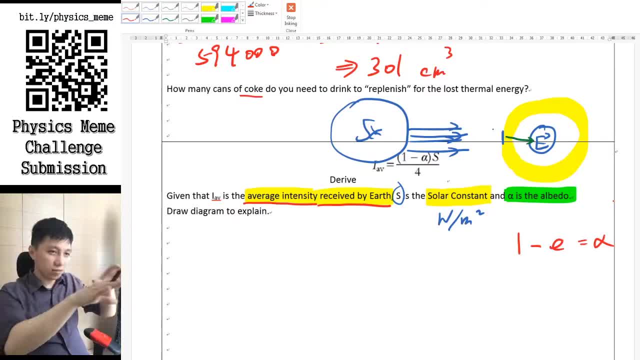 albedo, But then this one in the derived work here is not going to be necessary, so you can put it aside. maybe you can put it in the data booklet and this might be useful for your homework later on. But then this is the idea of the albedo itself. 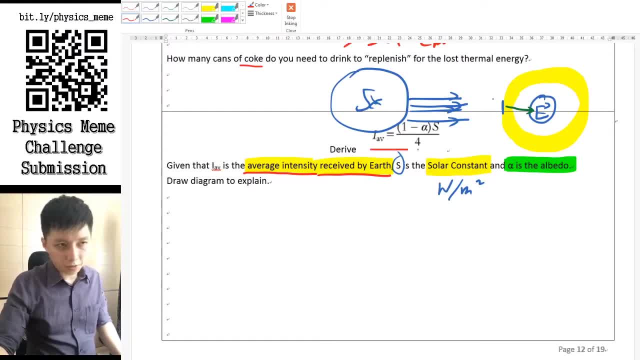 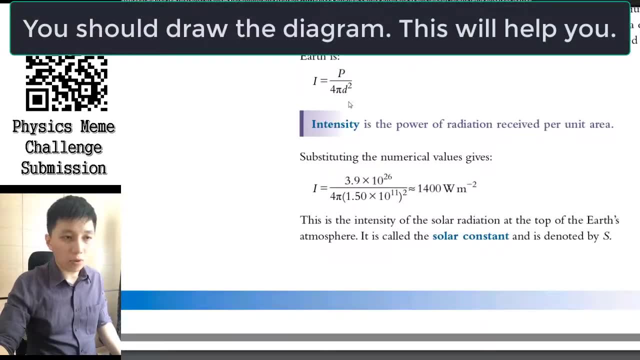 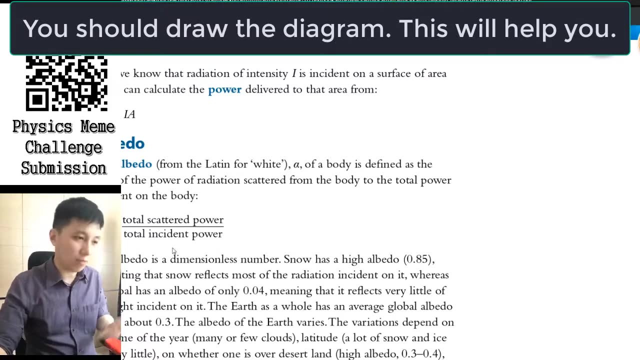 That should be all you need to know for deriving this equation, and if you really need to know more hints, of course you're welcome to read more of the test book, on page 332 and 333.. If you want more fun, more excitement, then maybe you can try. 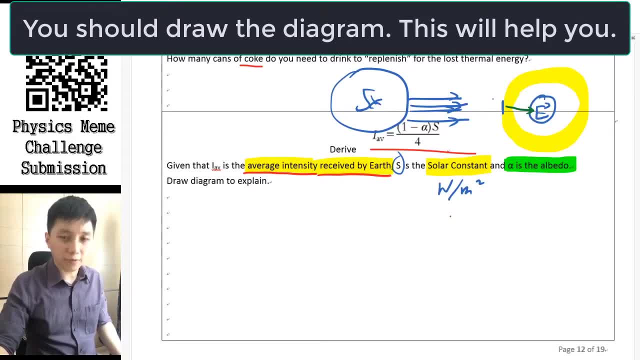 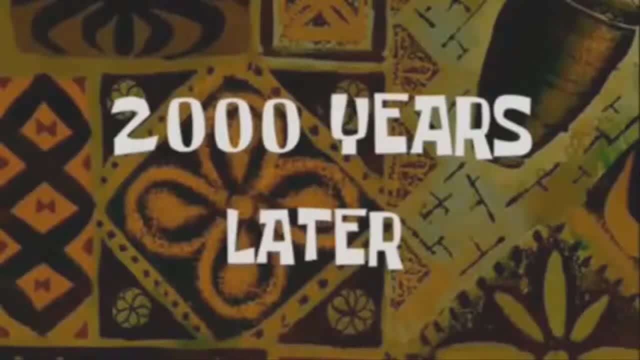 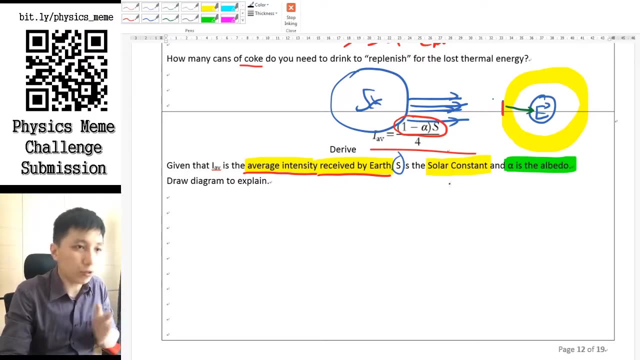 to start deriving the equation yourself. So pause the video now, try it out and I'll show you how we can do it. Alright, so there are actually two parts of doing your derived work here. So the first part is very easy, which is just by thinking of the definition of albedo. 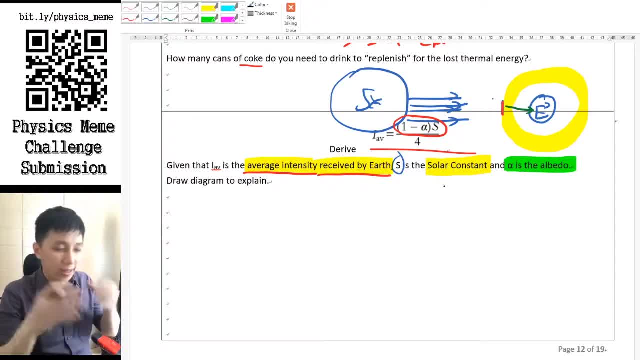 So, once again, albedo is how much, in terms of ratio, the light got reflected away. So the first part is very easy, which is just by thinking of the definition of albedo. So, once again, albedo is how much, in terms of ratio, the light got reflected away. So first part is very easy, which is just by thinking of the definition of albedo. So, once again, albedo is how much, in terms of ratio, the light got reflected away. So the first part is very easy, which is just by thinking of the definition of albedo. So, once again, albedo is how much, in terms of ratio, the light got reflected away. 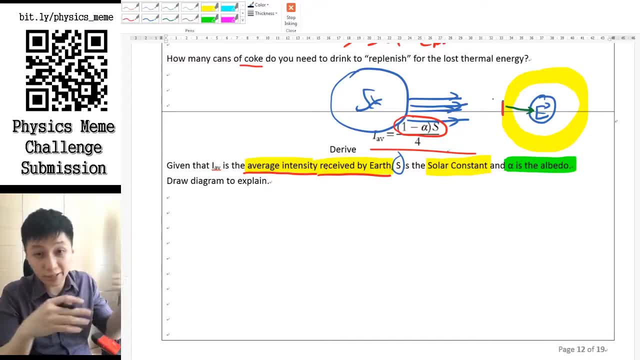 So if you want to find out how much is being retained or transmitted through it, then it will simply be the remaining, so 1 minus Alpha or the ratio. So that means you find out how much is going through it. And since at the top of the atmosphere the light intensity 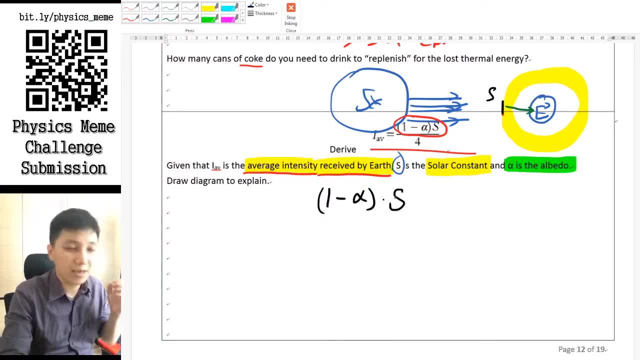 from the sun is actually S, so we just have to multiply S here, so then we can find out how much of the intensity from the sun can go through, go through the atmosphere. this is the first part, and this is easy, for the next part is slightly harder, and you have to think of the geometry of the whole. 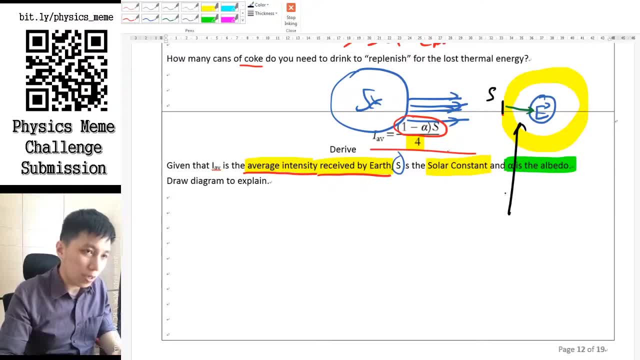 process. so let's try to zoom in here, and so if you try to redraw the earth again, it is a sphere and the sunlight, after passing through the atmosphere it should still be light parallel to each other and shining onto the earth. although in fact there should be some refraction happen in the atmosphere, we ignore it. 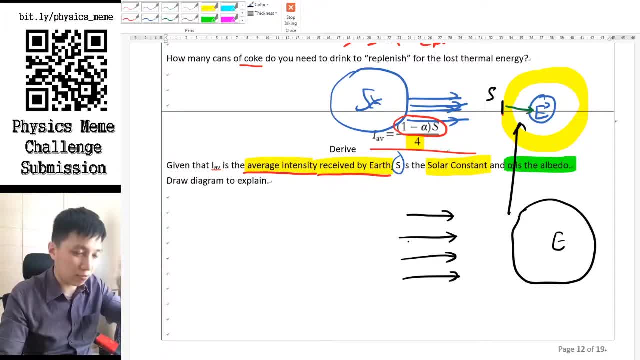 we just assume it just goes straight, okay in this, in this calculation. so if you try to think about, the light that got received by the earth is actually not on the spherical area, but then it comes in a circle, actually right, because only within that circle the light can actually illuminate onto the earth. so 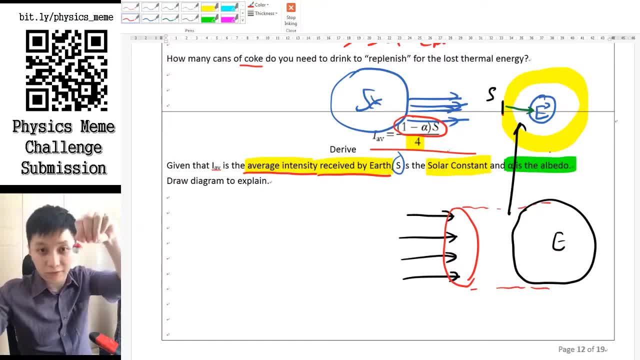 the idea is like: here I got a ball, which is one of my favorite here, and if you imagine there are lights shining through it, the one at the back right would be dark. this is like why we have night and daytime when the earth is rotating, and so no matter which. 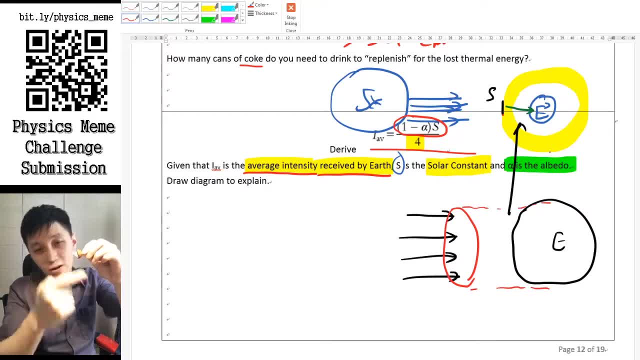 direction you are, there must be. only half of the earth is being illuminated by the sunlight, but then if you think of the light is going in a parallel light, then a circle of light, right, that particular area would have the light literally illuminate onto a sphere. so that's why in our calculation we should only account. 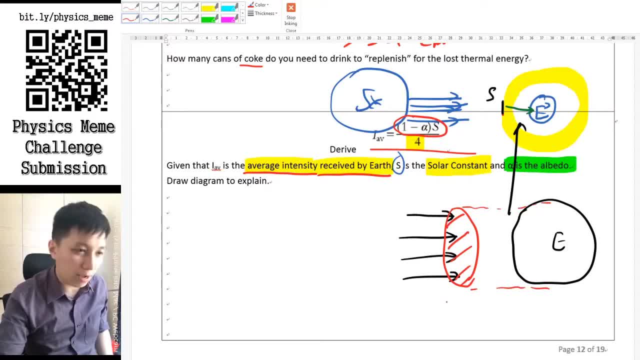 this circular area which, by pi, R square, and for the R we will be using the earth radius, because that is how it get defined, because if the earth gets bigger, then this circle will also get bigger as well, but then it is 2d instead of 3d, or 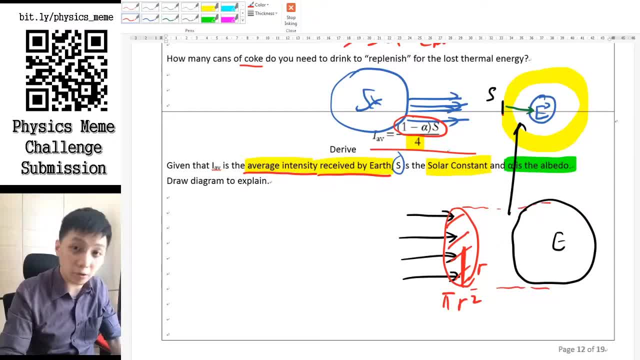 whatsoever, and so this can tell you the power that actually comes from the Sun. however, when the earth try to receive this power, it will be shared by a larger area, because this is 3d, so the area is much larger, and so by calculating this spherical area, we'll use the whole earth right, because we are trying to 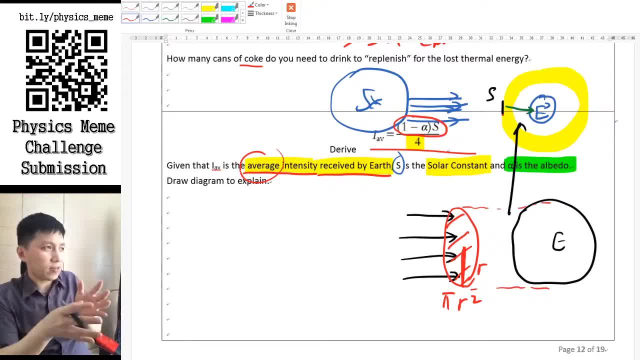 calculating the area of the earth and we are trying to calculate the area of the earth. because we are trying to calculating the area of the earth and we are trying to calculate the area of the earth and we are trying to calculate the area of the earth and we are trying to calculate the area of the earth and we are just being. 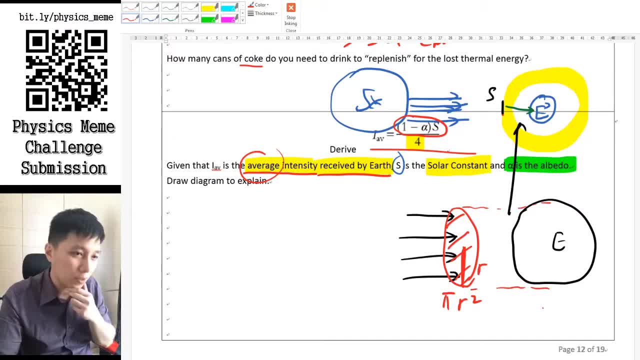 very En wt, Но我們聽這些意味著所有家母. WHO Barnett, quatre Austria alcoholics, both Nuria, Yes, please. so that's gonna be 4 pi R squared for the. so I think now it's very obvious why there is a divide. four, you know E. 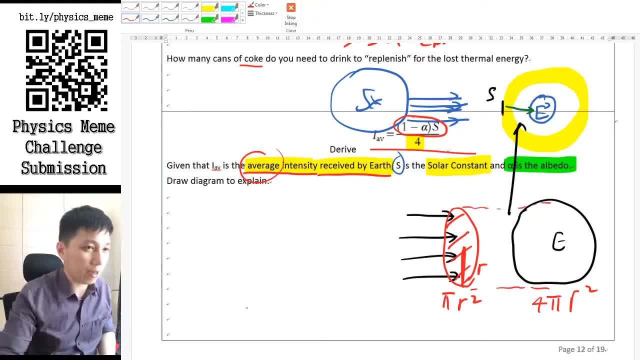 so that's gonna be 4 pi R squared for the spherical survey area. so I think now it's very why there is a divide for in your equation, because we could now evaluate the average intensity to be, of course, one minus alpha bracket s, that is, how much light intensity remained after getting. 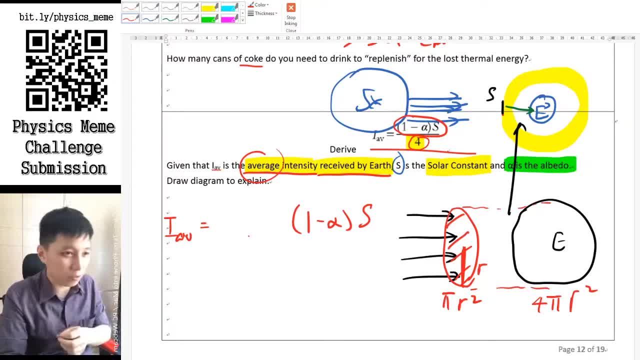 through the atmosphere. when we try to calculate is powered, then we can find it is pi R square, because after we multiply that with area, then we find power once again. the equation is: I use a P over a, so if you multiply a with intensity, then we are now finding its power. however, we still want to keep it as intensity, so 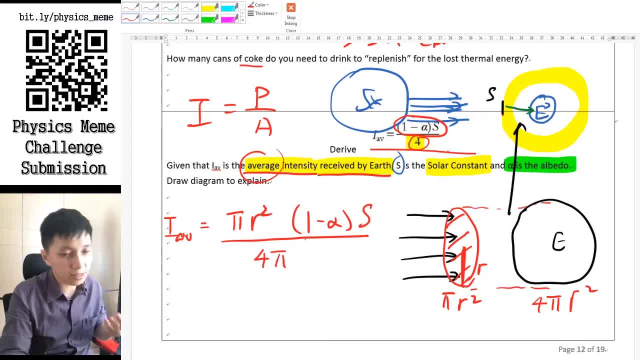 that's why we divide the area once again. but that, since is shared by the whole earth in spherical shape, then we will be 4 pi R, 4 pi R squared. so that is why, once again, these got cancel out and leaving you with the number of. 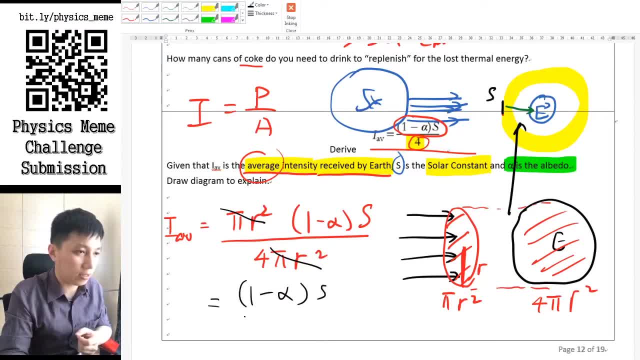 four down below. all right, so that's, it's exactly the reason. and in again in your exam, probably you'll be asked to do this yourself, because you don't have the formula in your data booklets. you cannot just recall it, you can't just say, oh, I. 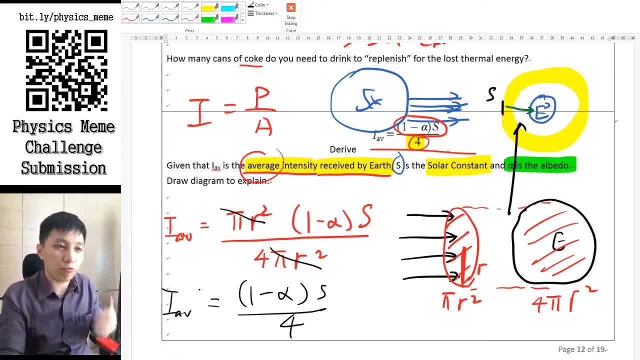 remember this equation. I just write it down. you can't do it, you have. you really have to show this and this in your working steps. lastly, you may ask me: hey, mr Wong, why do we bought this? because this is not, probably not even representable by the actual intensity. 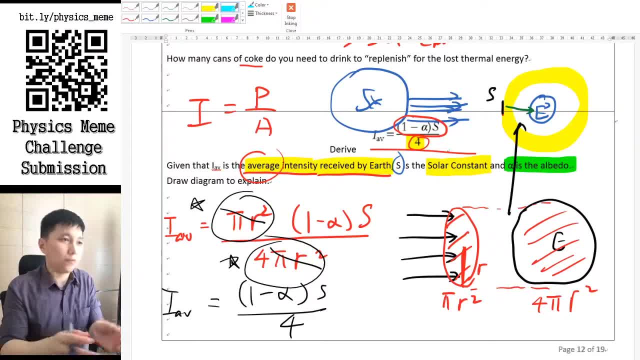 you receive on a spot on earth because it's taking the average. my answer is, or my explanation would be: yes, all right, it account for both day and night. so if you really want to account for only the days, then you can times it by two, right? that's one thing. the second thing is: people in the past may use this equation. 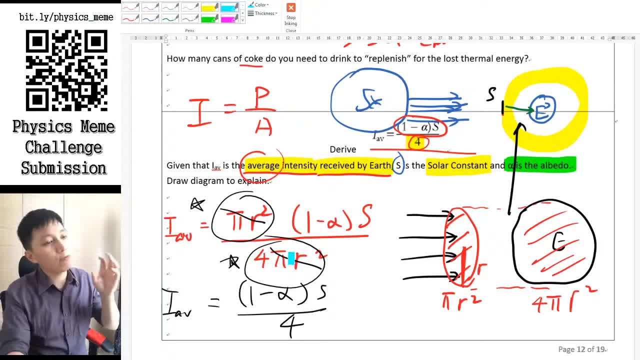 to verify the relationship between the parameters, and we may even use the number that we measure to calculate some other things, for example, in fact, in this equation, the one that is the easiest to measure, it's probably this instead: right, because this is simply you, if you have some sort of 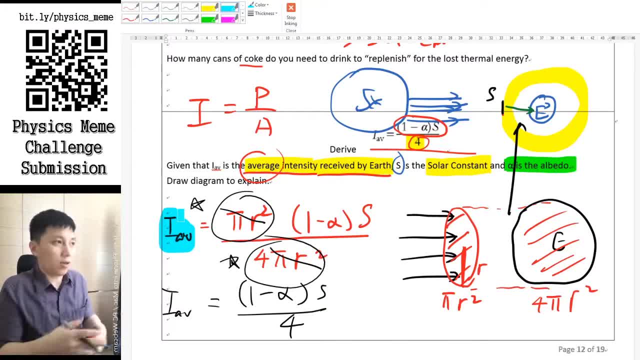 measurement tool like a light intensity meter, then you can simply measure whatever at your spot, at your location- Hong Kong, or whatever, New York, whatever is light intensity, and then you can use that to calculate some other things. so let's say, if you already know the not necessary earth radius, because you can. 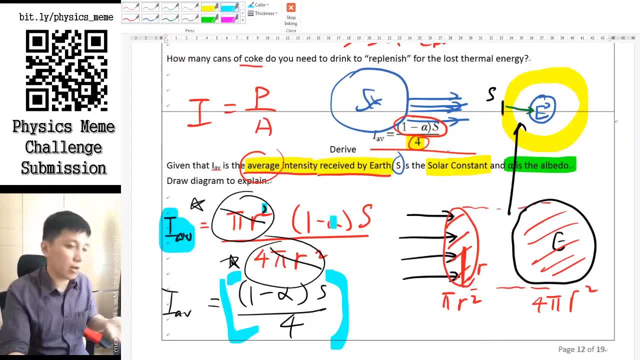 see in the equation, there's no earth radius here, but if you know somehow the solar constant, then you can use these two number, this number and this number, to calculate the albedo of the atmosphere. so maybe by using that we can calculate the different things, maybe the thickness of the atmosphere, etc. which. 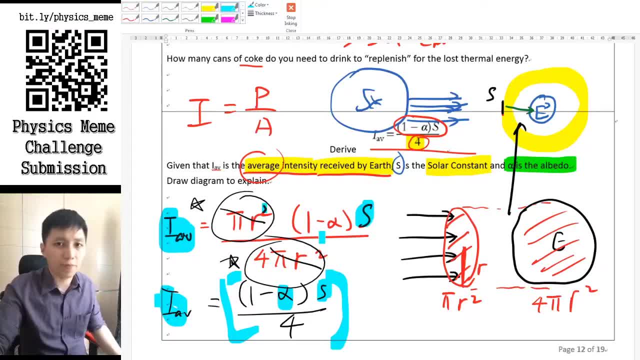 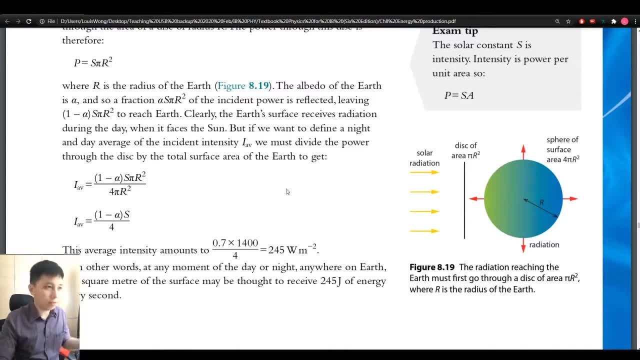 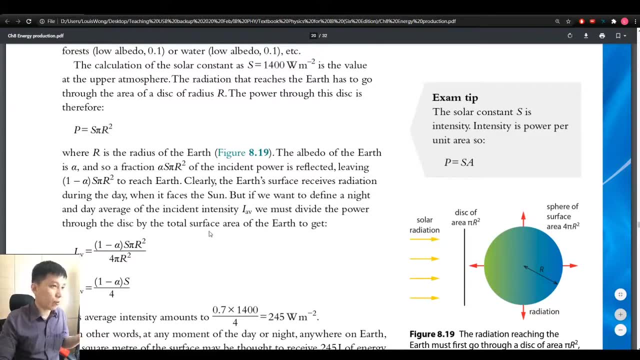 may be useful for our investigation in the future. second, lastly, if you try to look at the textbook calculation, if you try to substitute all the numbers- which of course you can do it as well- by s equal to 1400 and albedo technique as 0.3, 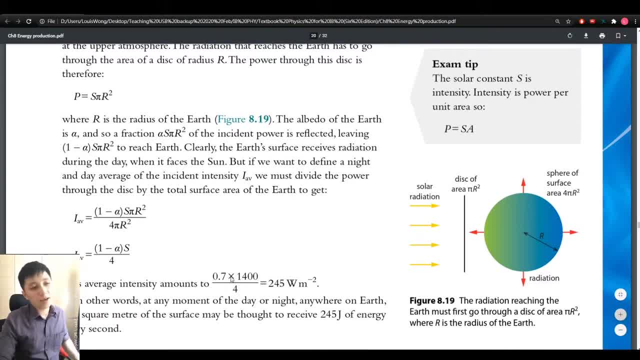 and so 1 minus albedo will be 0.7, and you'll be able to find the light intensity received by the earth to be 245 watts per meter square. and so, okay, what do you think about this number? then? if you try to think about, when you try to operate a 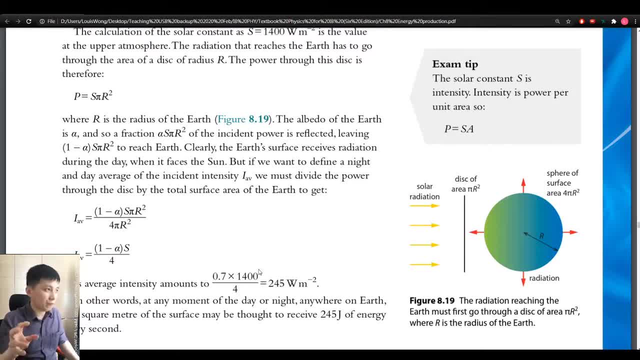 certain electrical appliance, it should also be a few, a few hundred watts as well. if you think of a light bulb, usually like the one that I have right now, it usually will be less than 100 watts. or you can go and check out the package of the light bulb that you are using. usually it's about 50 or 80 or at. 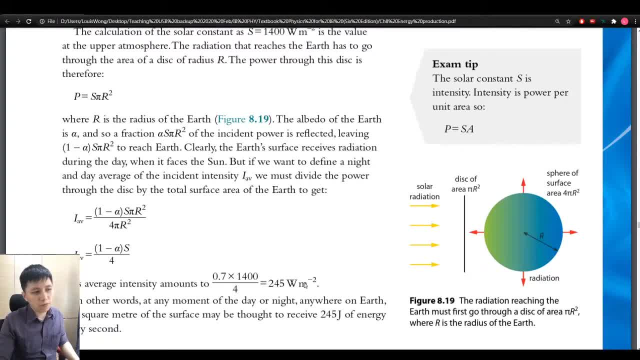 most 100 watts per light bulb. so if you think about the fact that if we human can harvest the light energy totally 245, then it's gonna be a lot. all right, we probably can't escape from using the fossil fuel, which would emit the co2 and 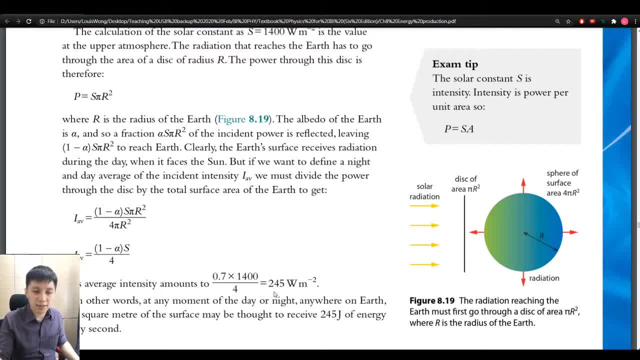 other greenhouse gases and make a gas that would emit the co2 and other greenhouse gases. and make a gas that would emit the co2 and other greenhouse gases. and make a gas that would emit the co2 and other greenhouse gases and make a planet a better place. so that is why there's a company called SolarCity. I'm planet a better place, so that is why there's a company called SolarCity. I'm planet a better place, so that is why there's a company called SolarCity. I'm not sure if you heard about that. it's not sure. if you heard about that, it's. 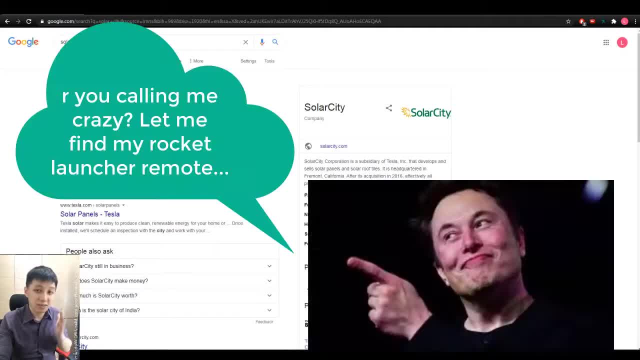 not sure if you heard about that. it's actually also by the crazy guy Elon Musk. actually also by the crazy guy Elon Musk. actually also by the crazy guy Elon Musk. all right, you can see here here Solar. all right, you can see here here Solar. all right, you can see here here. Solar City is a subsidiary of Tesla, Tesla. City is a subsidiary of Tesla. Tesla City is a subsidiary of Tesla. Tesla again is the electric car company, and so again is the electric car company, and so again is the electric car company. and so, other than the boring machine, the SpaceX, other than the boring machine, the SpaceX. 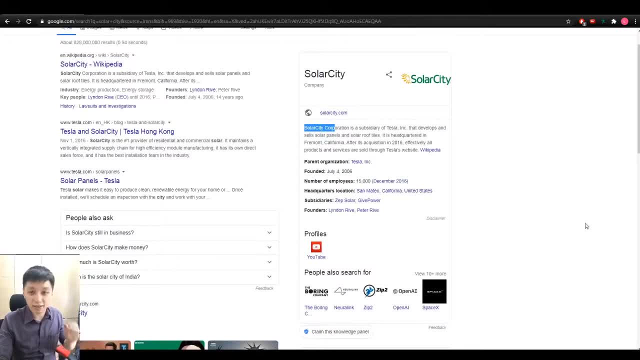 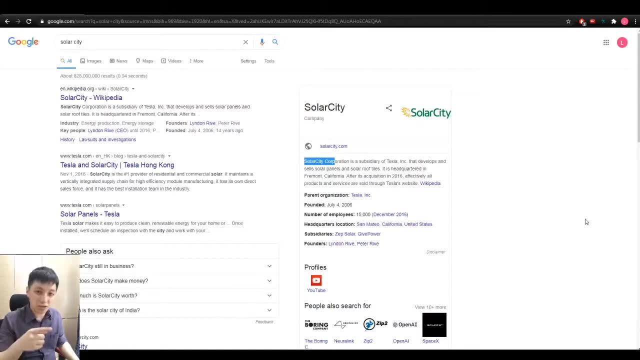 other than the boring machine: the SpaceX, Tesla, and recently the neural link for Tesla, and recently the neural link for Tesla and recently the neural link for like a machine, like a chip that put into. like a machine, like a chip that put into. like a machine, like a chip that put into your brain, Elon Musk, actually long ago. 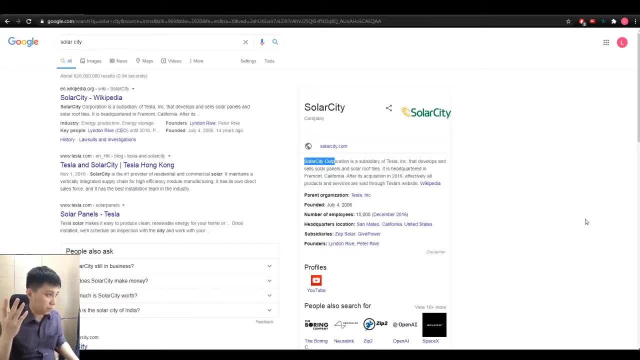 your brain, Elon Musk, actually long ago. your brain, Elon Musk, actually long ago, has already thought of the future, or as has already thought of the future, or as has already thought of the future, or as a vision that human would eventually, a vision that human would eventually a vision that human would eventually rely on the solar powered. all right, 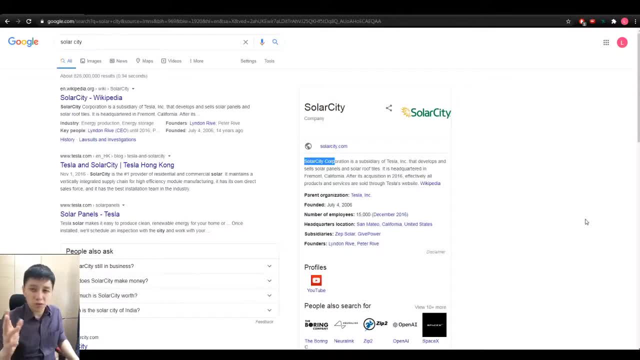 rely on the solar powered, all right. rely on the solar powered, all right, other than photofill. or maybe for new other than photofill, or maybe for new other than photofill, or maybe for new care is not really that versatile, or it. care is not really that versatile, or it. 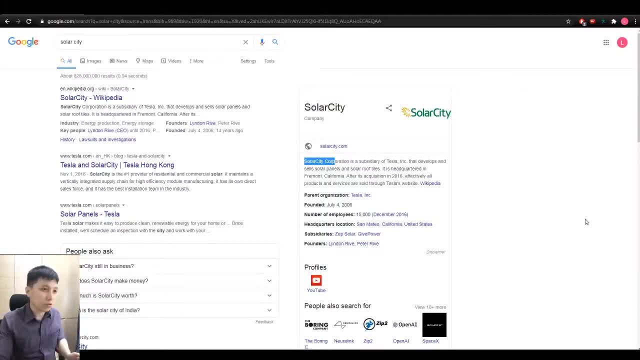 care is not really that versatile, or it takes a lot of effort to monitor, so takes a lot of effort to monitor, so takes a lot of effort to monitor. so solar panel is actually one of our. solar panel is actually one of our. solar panel is actually one of our future goal, and in a lot of different. 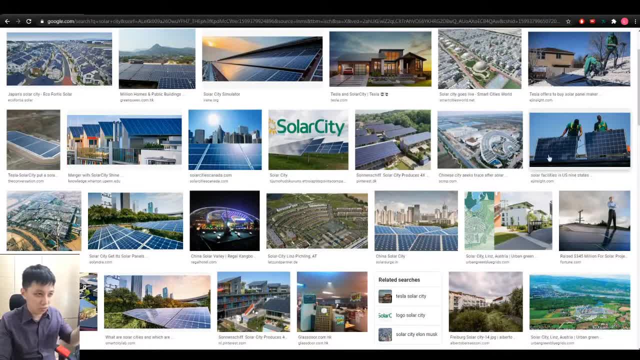 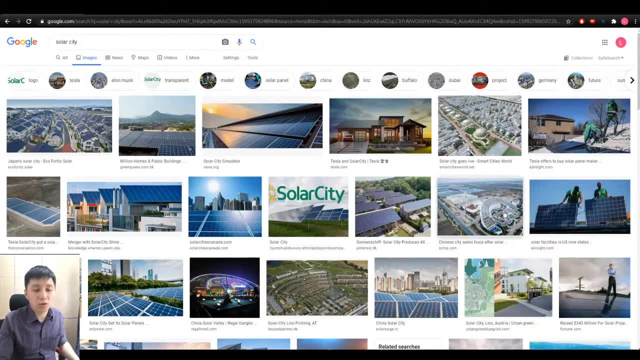 future goal and in a lot of different future goal and in a lot of different countries. we have already adapted into countries we have already adapted into countries we have already adapted into using this green energy, renewable energy, using this green energy, renewable energy, using this green energy, renewable energy, and so we, hopefully, will see more of the. 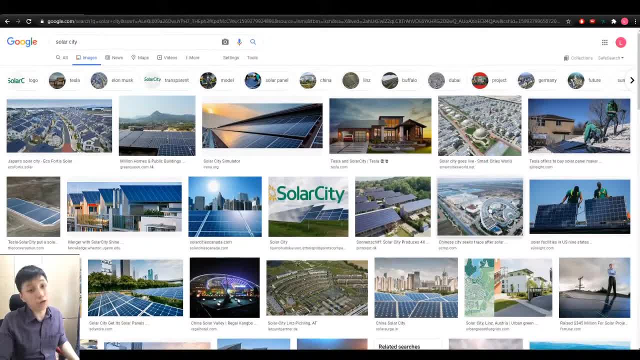 and so we hopefully will see more of the and so we hopefully will see more of the different countries would get into this, different countries would get into this, different countries would get into this and again, hopefully, to reduce the amount, and again hopefully to reduce the amount and again, hopefully, to reduce the amount of co2 emission. really, really. lastly, if 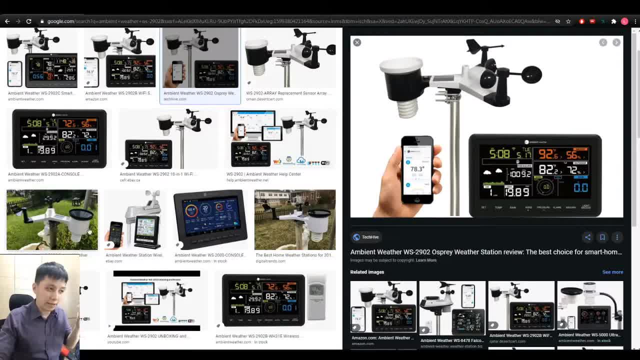 of co2 emission really really. lastly, if of co2 emission really really. lastly, if you are sitting at my school- that I'm you are sitting at my school, that I'm, you are sitting at my school, that I'm teaching- you know that we have a mini. 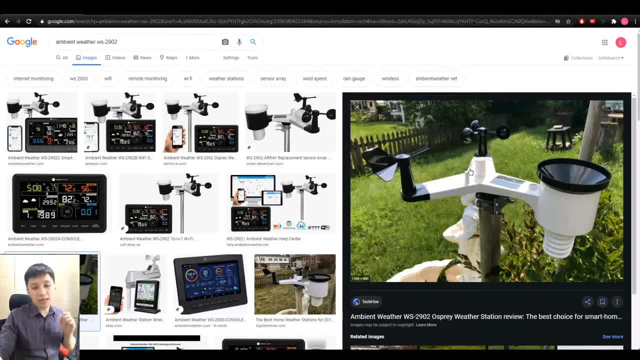 teaching. you know that we have a mini teaching. you know that we have a mini weather station. that is something like weather station. that is something like weather station, that is something like that, and it collects weather data, all that. and it collects weather data, all that. and it collects weather data all right, including temperature rain. 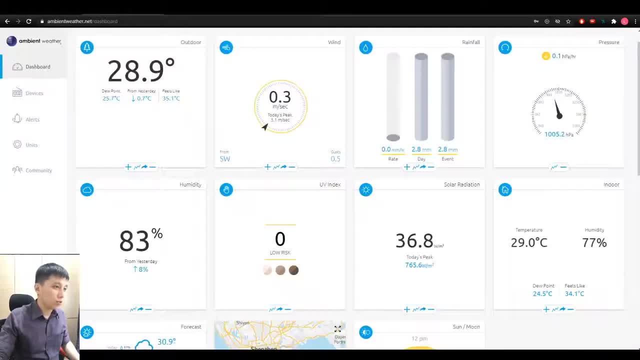 right including temperature, rain right including temperature, rain, raindrop or wind speed etc. so you can raindrop or wind speed etc. so you can raindrop or wind speed, etc. so you can actually access to those data through actually access to those data, through actually access to those data through the link here. I'll put the link in: 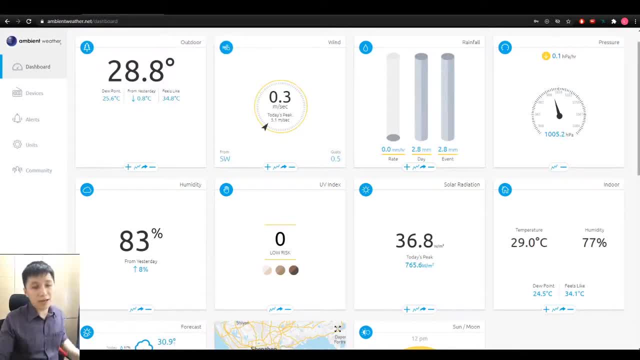 the link here. I'll put the link in the link here. I'll put the link in description below and the most important description below and the most important description below and the most important thing that I would like to see and link, thing that I would like to see and link. 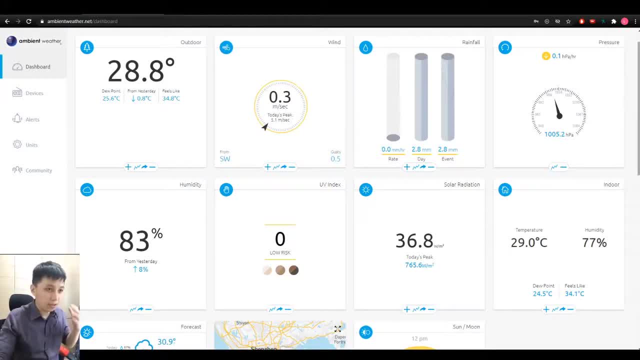 thing that I would like to see and link it with our topic right now is the solar it with our topic right now is the solar it with our topic right now is the solar radiation. so now you can actually see radiation. so now you can actually see radiation. so now you can actually see that the solar radiation at the time. 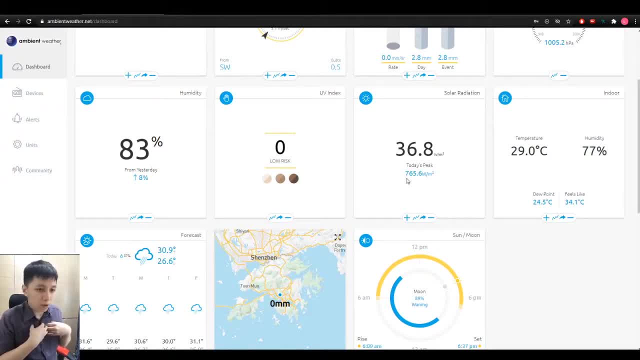 that the solar radiation at the time, that the solar radiation at the time, right now, now, what I'm doing. this video right now now, what I'm doing. this video right now, now, what I'm doing this video is on 6th of September, around 4 pm, so 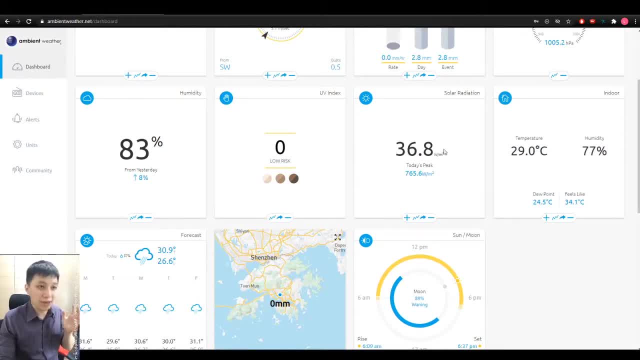 is on 6th of September around 4 pm. so is on 6th of September around 4 pm. so you can see that the solar radiation is. you can see that the solar radiation is. you can see that the solar radiation is actually 36.8 watts per meter square. so 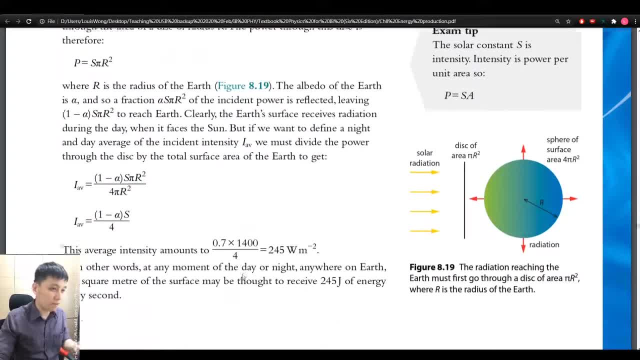 actually 36.8 watts per meter square. so actually 36.8 watts per meter square. so it's actually way, way lower than the one. it's actually way, way lower than the one. it's actually way, way lower than the one that you have from the test also 245 and 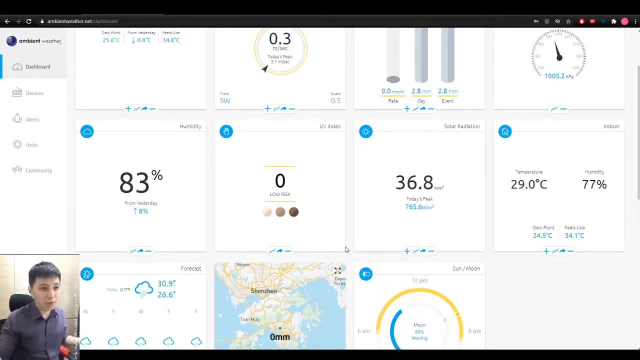 that you have from the test also 245, and that you have from the test also 245, and that is something to do with the cloud. that is something to do with the cloud. that is something to do with the cloud, with the different weather, however you, with the different weather, however you. 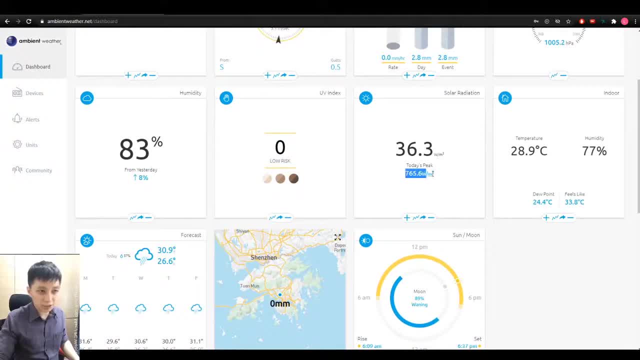 with the different weather. however, you can see that interestingly, you can see. can see that interestingly, you can see. can see that interestingly, you can see: the peak is that the peak of today is the peak is that the peak of today is the peak is that the peak of today is actually 700 something. so I think that's. 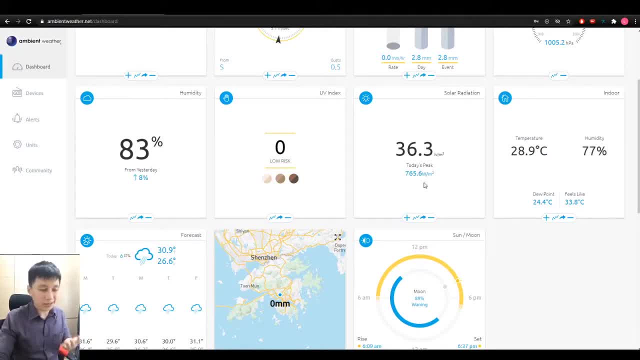 actually 700 something. so I think that's actually 700 something. so I think that's why we would need to take the average, why we would need to take the average, why we would need to take the average, because that is the most important. it's because that is the most important it's. 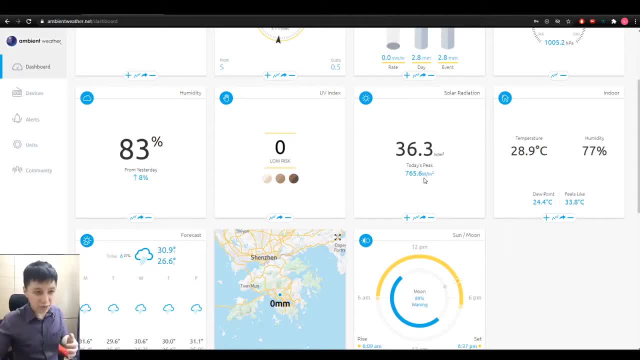 because that is the most important. it's not about just this moment or in the. not about just this moment or in the, not about just this moment or in the next moment when this is a peak, but next moment when this is a peak, but next moment when this is a peak, but then it's more about the average. you. 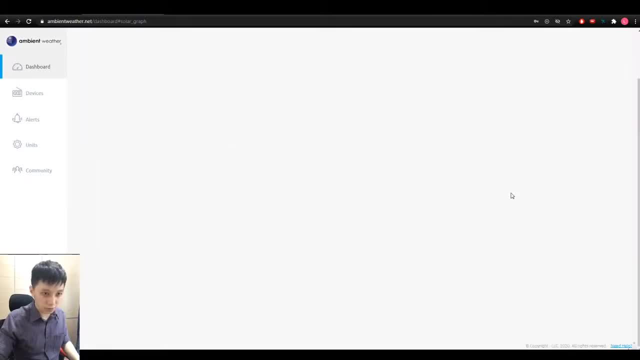 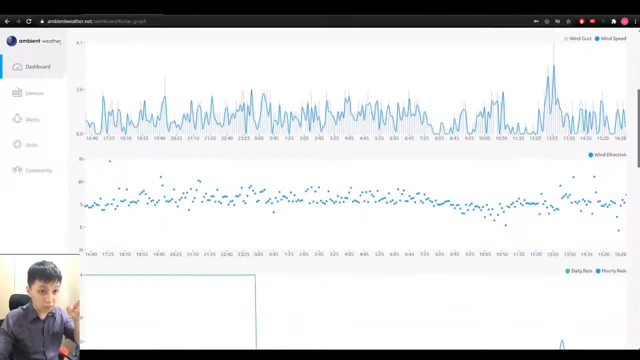 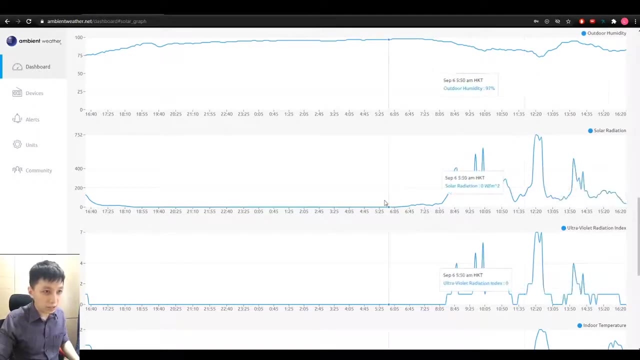 then it's more about the average. you, then it's more about the average. you get wind direction rain pressure. get wind direction, rain pressure, get wind direction, rain pressure. humidity, solar radiation. so here you go. humidity, solar radiation, so here you go. humidity, solar radiation. so here you go. okay, so you can see that when it is at. 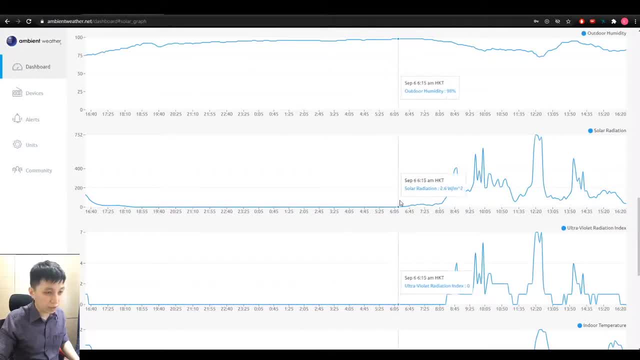 okay, so you can see that when it is at, okay, so you can see that when it is at the night before sunshine, it is, you know, the night before sunshine, it is, you know, the night before sunshine, it is, you know. zero, obviously, because there's no. zero, obviously, because there's no. 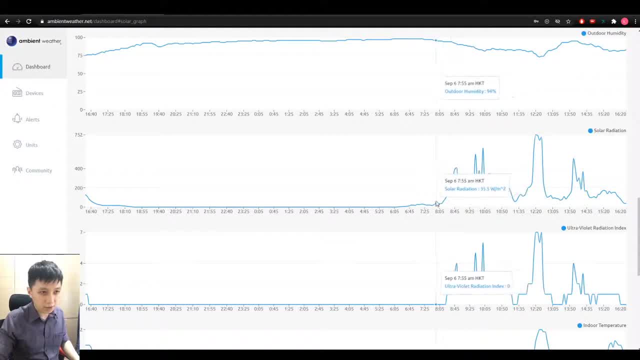 zero, obviously, because there's no sunlight at all, but then later on when sunlight at all. but then later on when sunlight at all. but then later on when it is around. I think around 7 am I. it is around, I think around 7 am I. 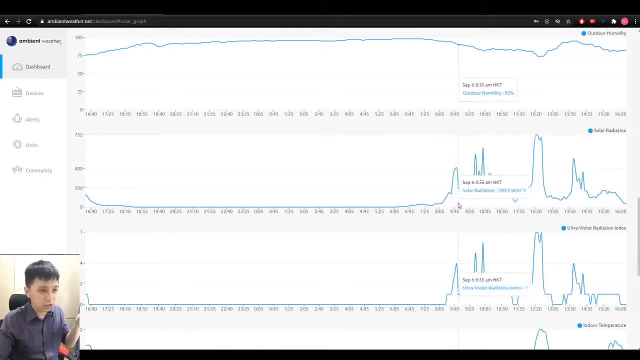 it is around, I think around 7 am. I guess a sunrise and there will be some guess a sunrise and there will be some guess a sunrise and there will be some sunshine on to the machine, the weather sunshine on to the machine, the weather sunshine on to the machine, the weather station itself, and so that's why I go up. 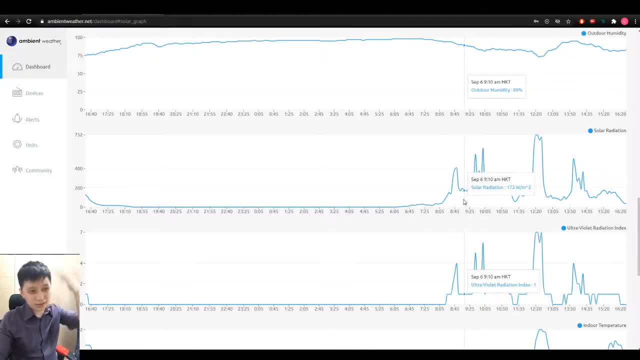 station itself, and so that's why I go up station itself, and so that's why I go up. but there are times, maybe there are, but there are times, maybe there are, but there are times maybe there are some cloud that covering the sunlight, some cloud that covering the sunlight. 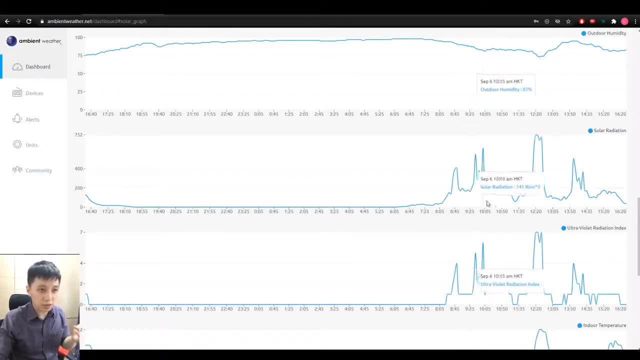 some cloud that covering the sunlight onto that machine, and so that's why it onto that machine and so that's why it onto that machine and so that's why it would drop way lower. so that's why kind would drop way lower. so that's why kind. 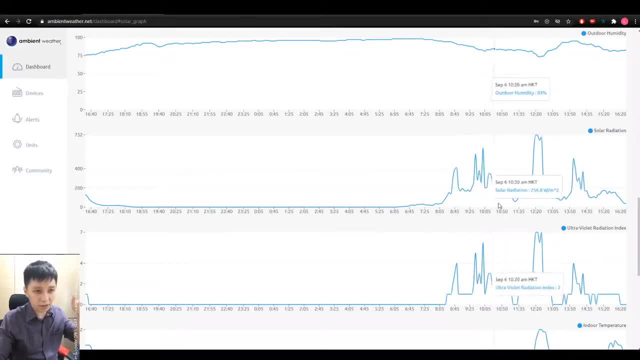 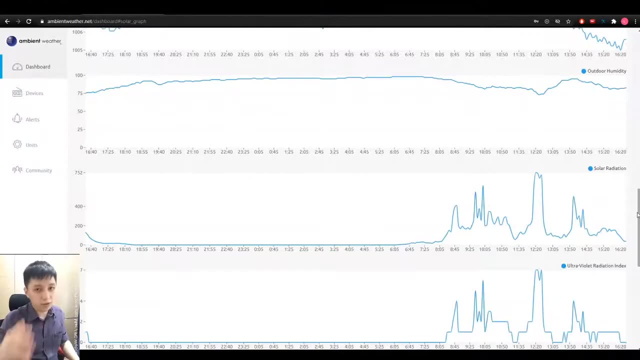 would drop way lower. so that's why- kind of fluctuate from- yeah, I think. 200 of fluctuate from- yeah, I think 200 of fluctuate from- yeah, I think 200. something is a really good estimation. something is a really good estimation. something is a really good estimation. really want you to take a look and try. 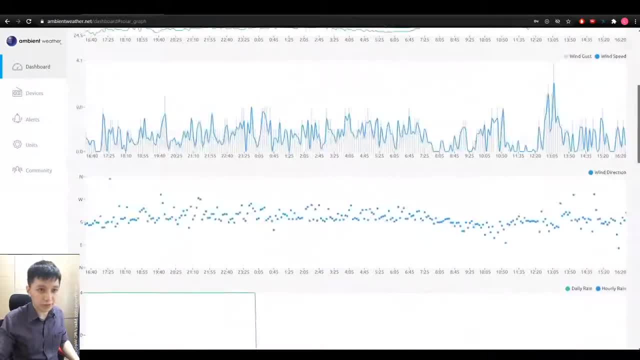 really want you to take a look and try, really want you to take a look and try to see the pattern is really interesting to see. the pattern is really interesting to see. the pattern is really interesting to see how different pattern in weather, to see how different pattern in weather. 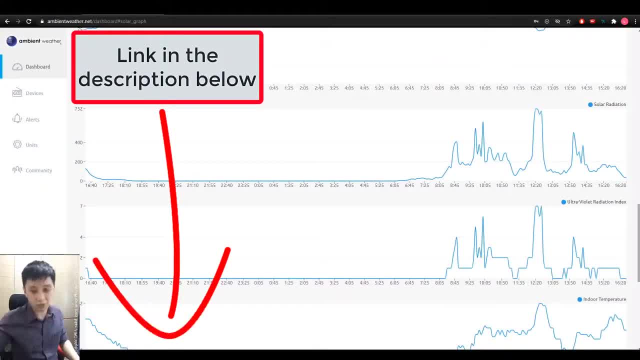 to see how different pattern in weather would correlate with each other, how and would correlate with each other, how and would correlate with each other, how and how that would change with the time. so how that would change with the time. so how that would change with the time. so, once again, I'll put a link in the